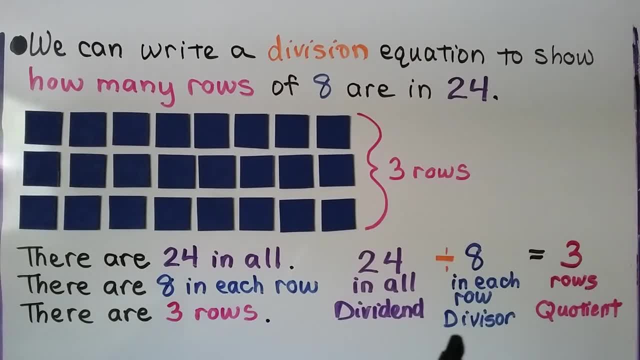 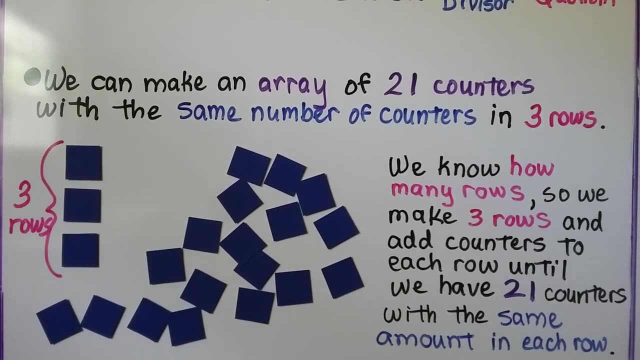 We have 24 in all. There's 8 in each row. We have 3 rows. 24 is our dividend, 8 is our divisor and 3 is our quotient. We can make an array of 21 counters with the same number. 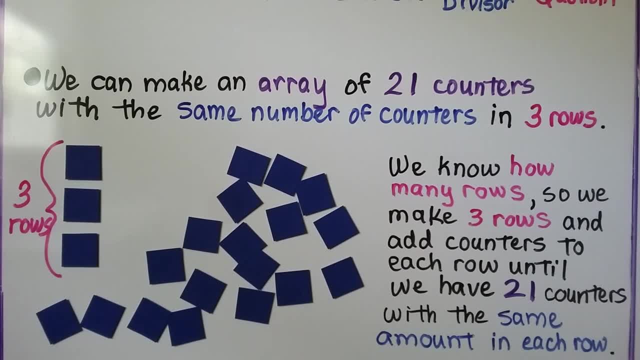 in three rows. We know how many rows we're supposed to have. there's three of them and we add counters to each row until we have 21 counters, with the same amount in each row. So we don't know how many are in the row, we only know that we 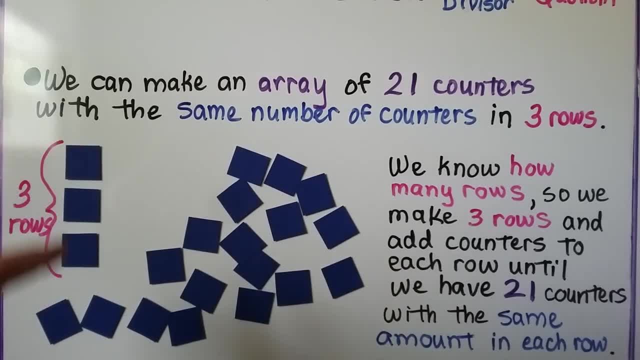 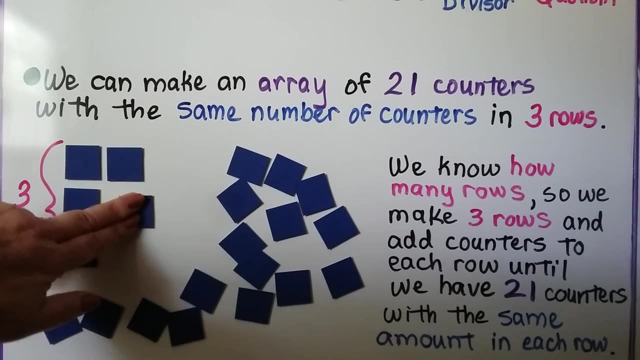 have three rows. So let's make a column for one row, two row, three rows, and let's keep filling them with the same amount of counters until we have 21.. So I have 21 counters in all, right here, and I can start putting them into rows. Now we have 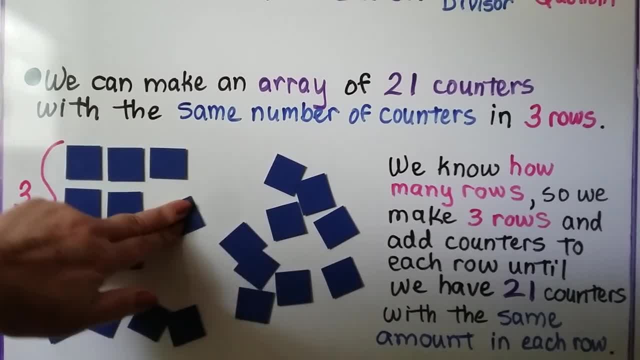 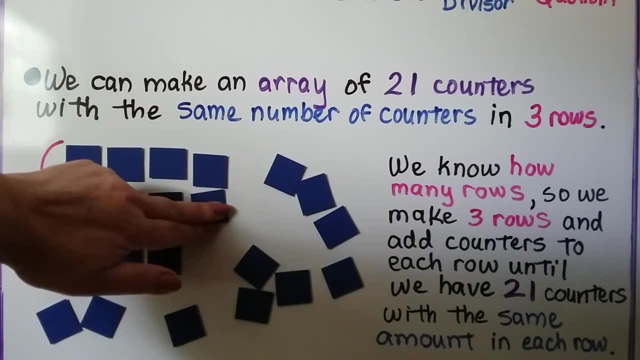 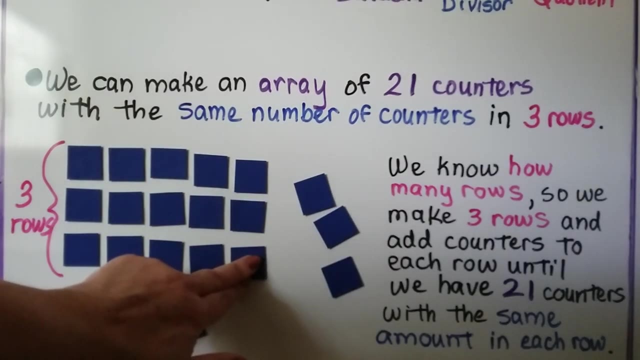 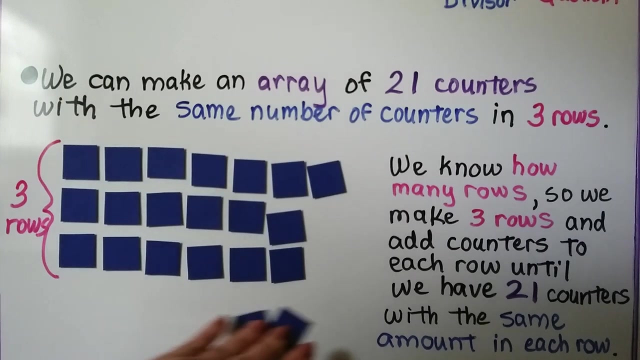 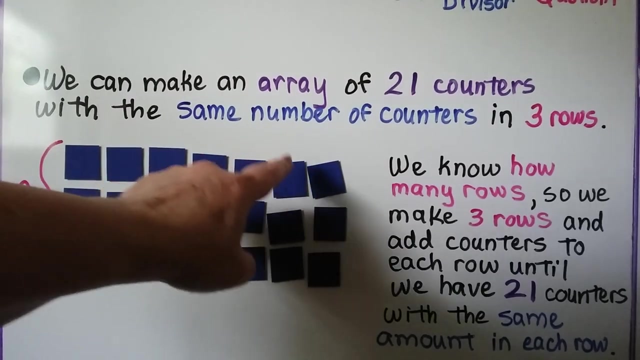 three rows with two in them. I have three rows with three in each row and we keep doing this equally until we have all of them with the same number in each row. Okay, Got a couple more, And one, two, three, four, five, six, seven are in each row. We 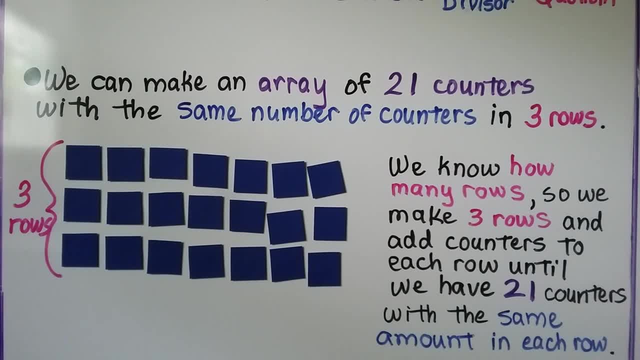 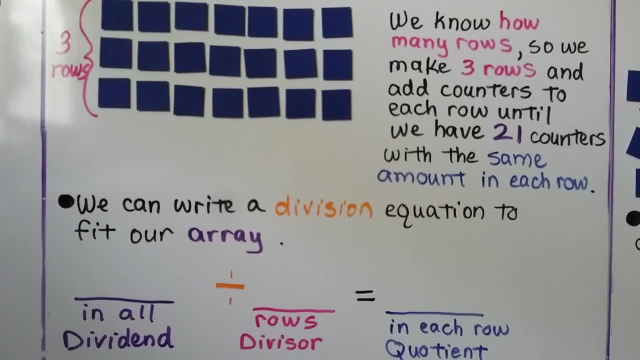 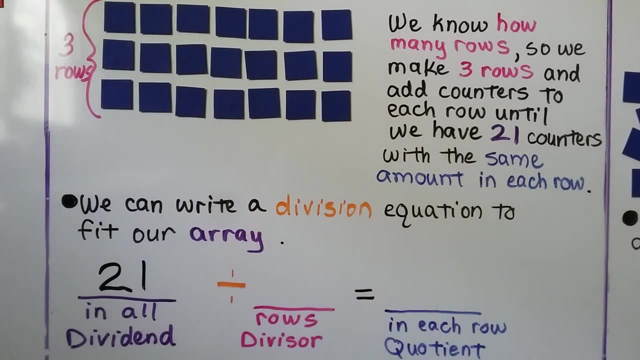 know that there's seven. 21 divided by three is equal to seven, So we write a division equation to fit our array. We know we have 21 in all. we know that there's three rows and we now know there are seven in. 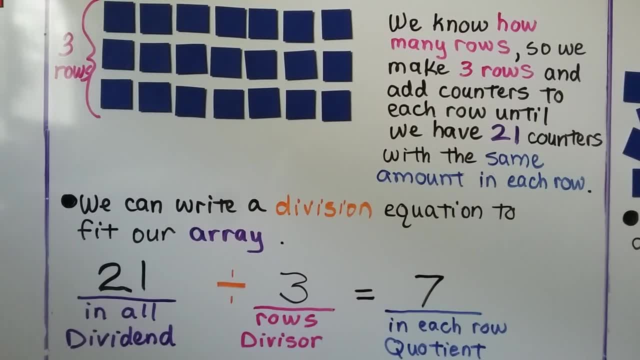 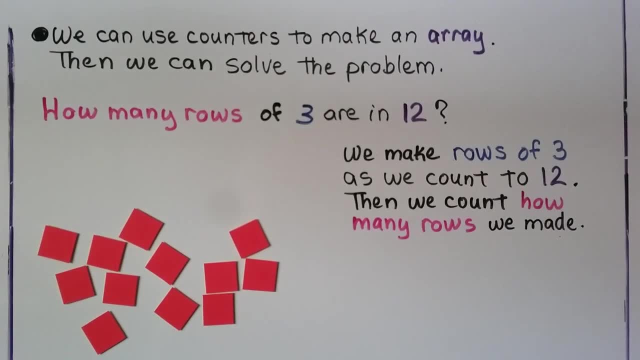 each row. 21 is our dividend, three is our divisor and seven is our quotient. our answer: We can use counters to make an array. then we can solve the problem: How many rows of three are in 12?? First thing we do is count out 12.. 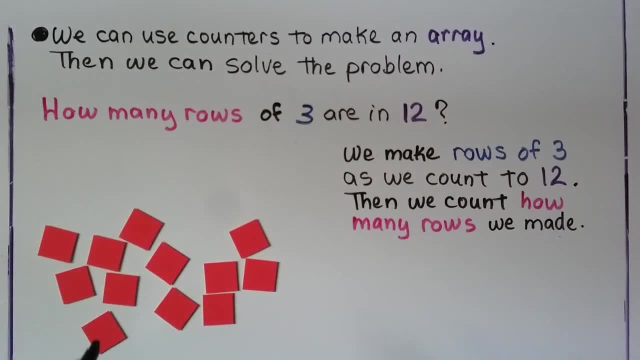 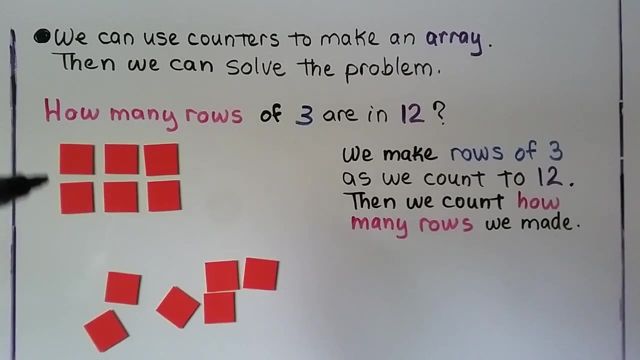 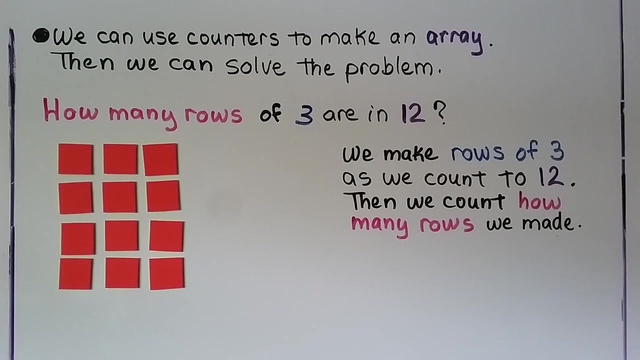 We make rows of three. so we're going to have three in each row And we count to 12.. Then we count how many rows we made. That's one row of three. Now we have two rows of three, three rows of three, four rows of three, Twelve in all. divided by three in each row is equal. 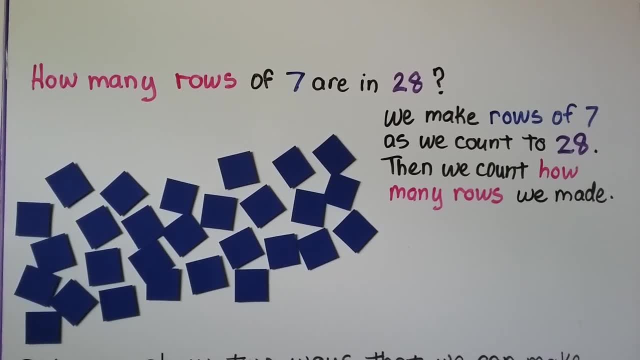 to four rows. How many rows of seven are in 28?? We make rows of seven as we count to 28.. So here we have 28 counters. We've already counted them out. We know there's 28. here We're going to make rows of seven. That's one row of seven, two rows. 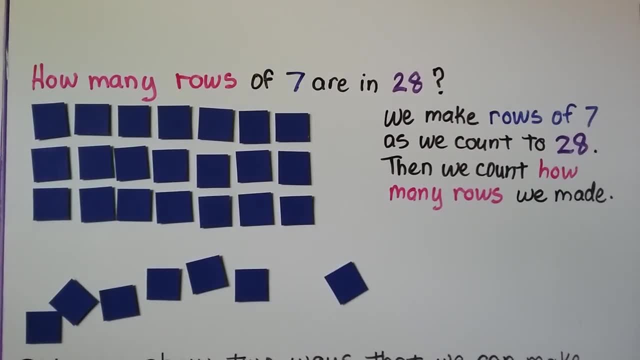 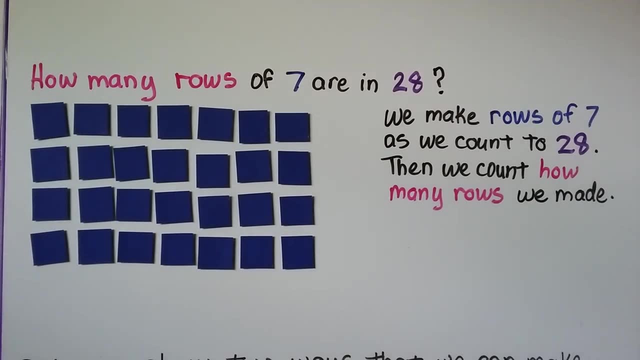 of seven, three rows of seven, four rows of seven. We count how many rows we have. We have made four. Our equation is 28,. that's how many we had in all divided by seven. that's how many were in. each row is equal to four, That's. 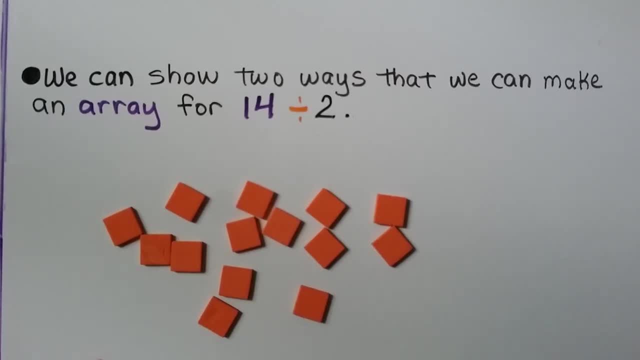 how many rows we made. We can show two ways that we can make an array for 14 divided by two. We can use two as how many rows we have, or the two could be how many are in each row. We count out 14 counters and we put them in two equal rows. 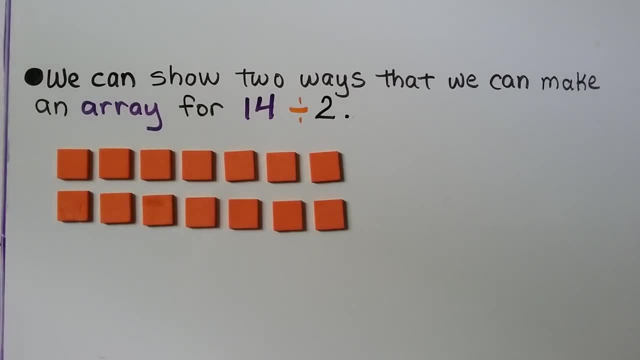 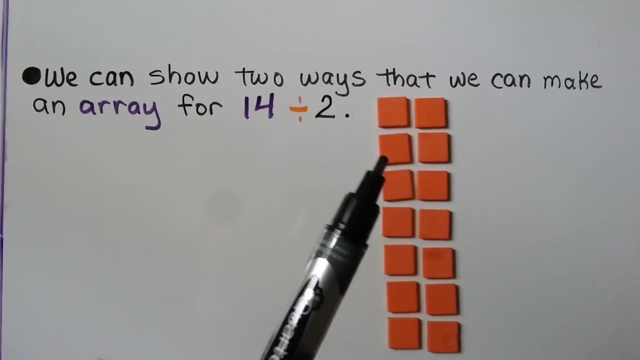 two equal groups. We see there's seven in each group, so 14 divided by two is equal to seven. We can also put two in each row. We still have 14 counters, but now we have two in each row and we've made one, two, three, four, five, six, seven rows. 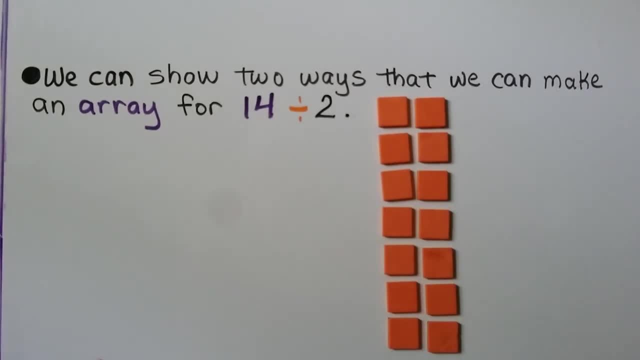 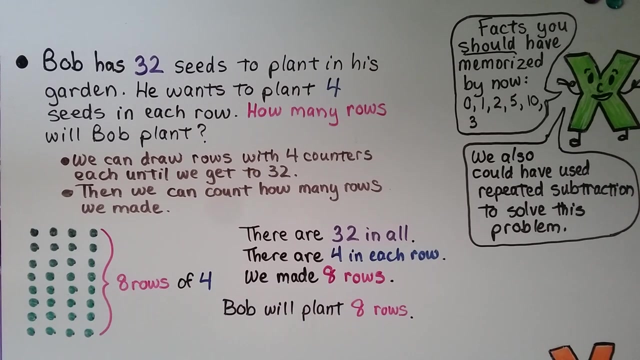 14 divided by two is equal to seven, So we can make them as two rows or two in each row. for the array, Bob has 32 seeds to plant in his garden. He wants to plant four seeds in each row. How many rows will Bob plant? We can draw rows with four counters each until. 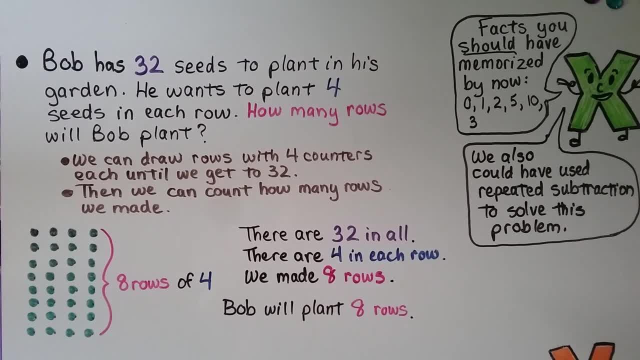 we get to 32.. Then we can count how many rows we made. We put four in a row, so that's four, and we keep drawing them: Five, six, seven, eight, nine, ten, eleven, twelve, thirteen, fourteen. 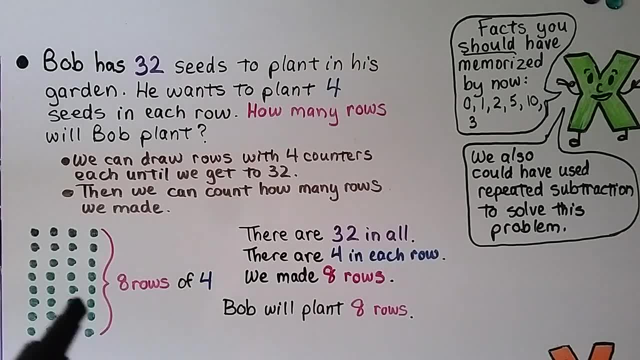 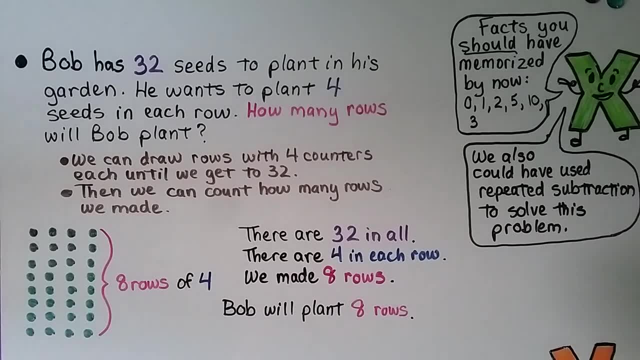 fifteen, sixteen, seventeen, eighteen, nineteen, twenty, Twenty-one, twenty-two, twenty-three, twenty-four, twenty-five, twenty-six, twenty-seven, twenty-eight, twenty-nine, thirty, thirty-one, thirty-two, With four in each row. then we count the rows One, two, three, four, five. 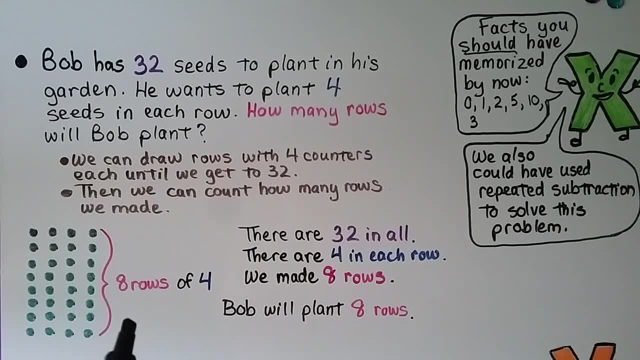 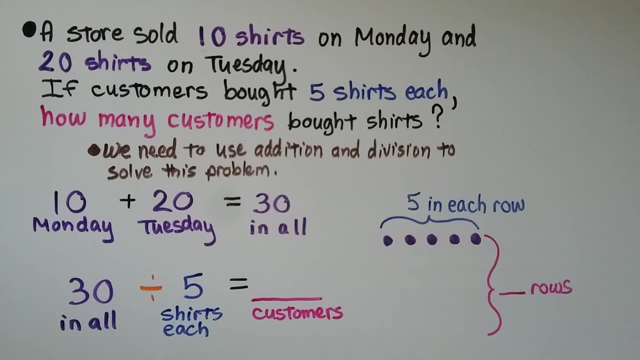 six, seven, eight, Two in all. there are four in each row and we made eight rows, So Bob will plant eight rows. A store sold ten shirts on Monday and twenty shirts on Tuesday. If customers bought five shirts each, how many customers bought shirts? So let's circle our important numbers first. 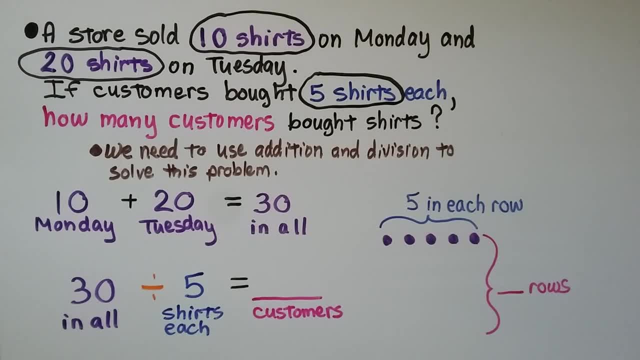 We can underline other important information. It's important that ten shirts were sold on Monday, twenty shirts on Tuesday and that customers bought five shirts each. We need to use addition and division to solve this problem. The first thing we need to do is: 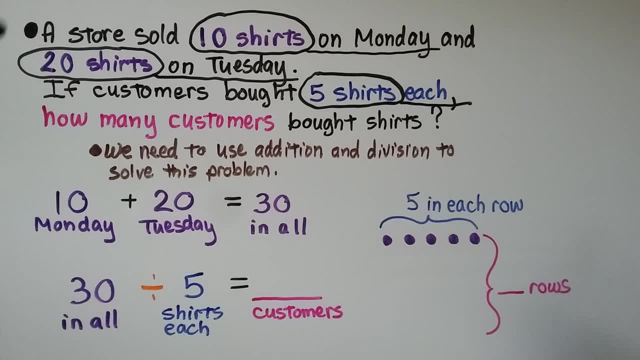 find out how many in all. We have ten shirts on Monday and twenty shirts on Tuesday. That's thirty in all. Then how many we have in all is going to be thirty. We know that customers bought five shirts each, so we're going to do thirty divided by five. So we've used addition to find how. 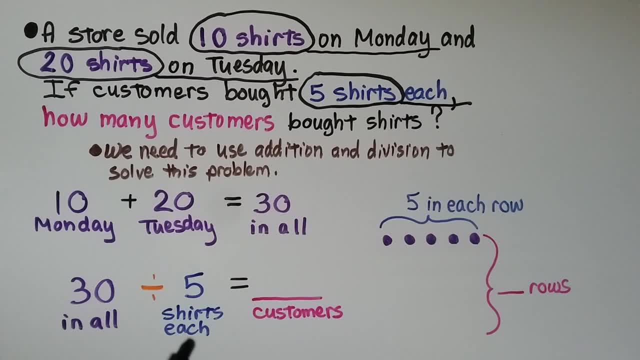 many in all. Now we're going to use division to find out how many customers bought shirts. We can make an array. There's five shirts for each customer and we can draw these until we get to thirty, with five in each row.